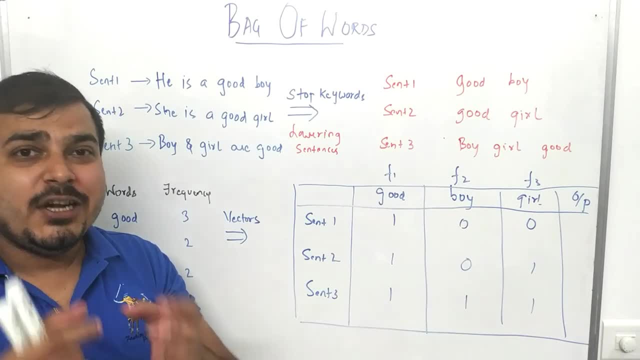 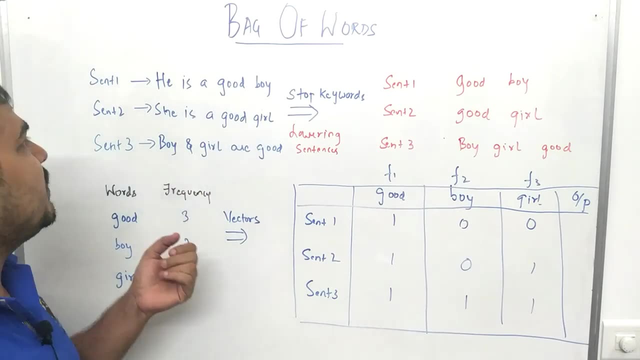 in that particular text data, I can just directly give it to my model. you know we need to convert that into some numerical format. We basically call it as vectors in case of NLP, natural language processing. Now suppose I have some examples over here in sentence one, sentence two, sentence three. 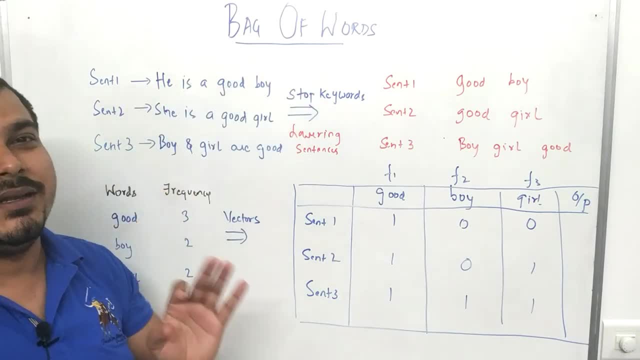 I have three positive statement and remember the output is 111 suppose. So the first sentence is he's a good boy. sentence two is she's a good girl. sentence three is boy and girl are good. okay, and always remember during text pre-processing we have to do some of the things like: first of all, we need 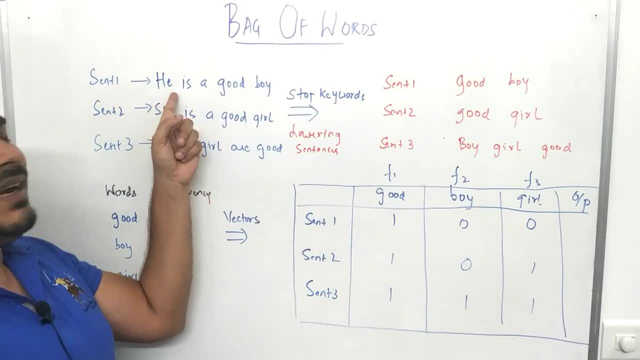 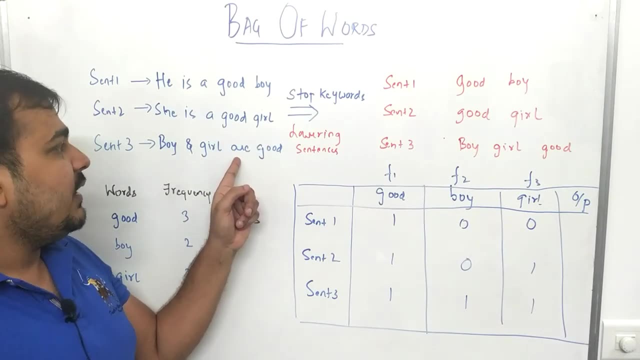 to lower the sentences because, understand, suppose over here capital HE is there, okay, and suppose somewhere in small HE may be there, right, and if I don't lower the sentence, both that particular word will be denoted in a separate way. So it is always good that you lower the sentences. 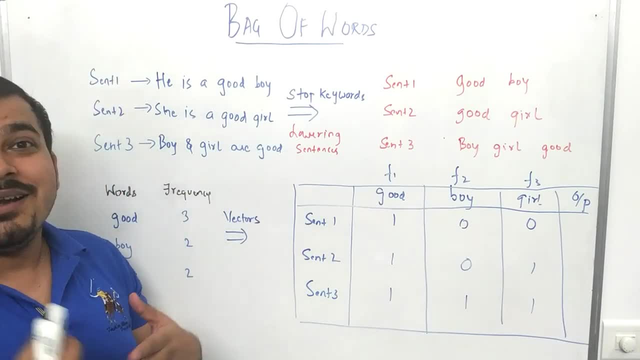 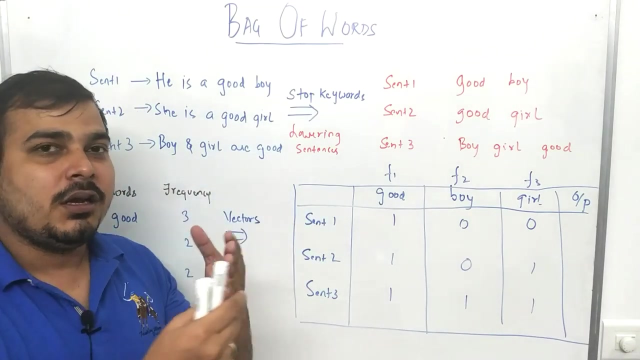 But yes, there are some scenarios, like suppose there is country's name, you know, like capital IN India or USA, capital US and small US, right, it will not match. So at that particular case you need you can actually consider that word in a separate list and later on you can just keep that particular. 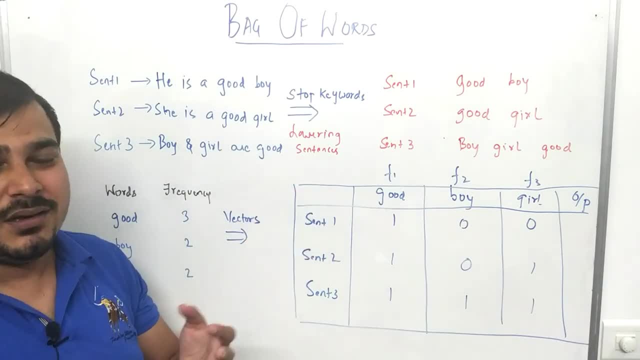 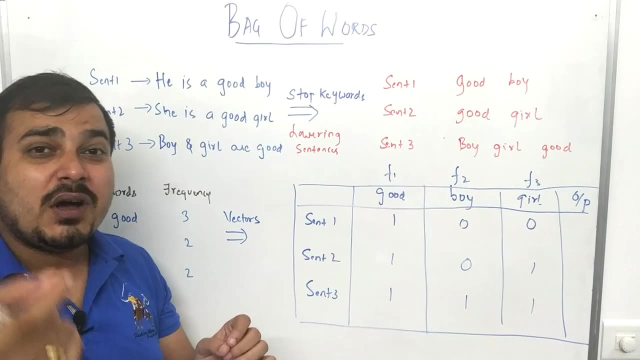 words and remaining all words, you can actually lower in the sentences. You can do that in normal in processing code season. So over here, first step is basically lowering the sentences. then what I can do is that I can also apply the sentence. So over here, first step is basically lowering the sentences. then what I can do is that I can also apply. 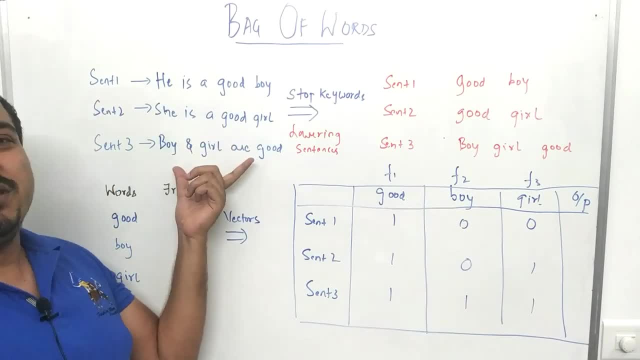 stemming and lemmatization. Over here I've just taken simple words. stemming and lemmatization is not required in this particular case, but you can do it, because in usual scenario you'll be having so many sentences Here. I've just taken an example of three sentences. Then we can also apply: stop. 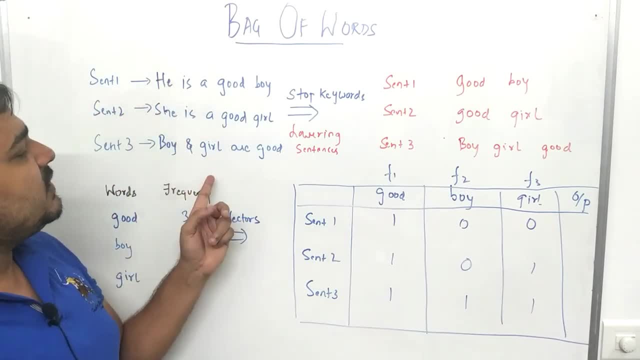 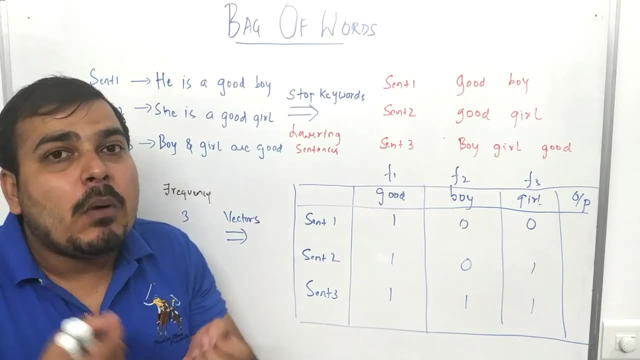 keywords. Now what is exactly stop keywords? Understand over here in this text data guys, we have so many words like is a, he, she are and right. these all are not important data, because I'll tell you why. Suppose I'm solving sentiment analysis, Suppose I'm solving sentiment analysis. Suppose I'm solving sentiment analysis. 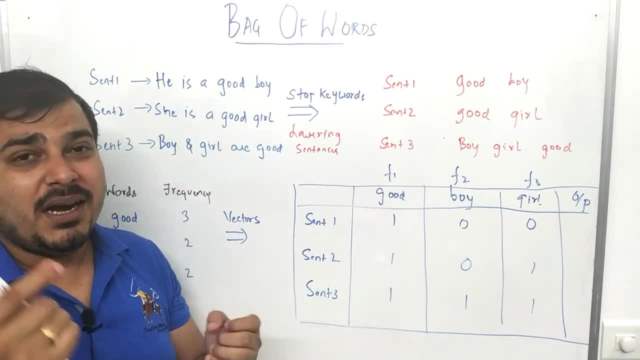 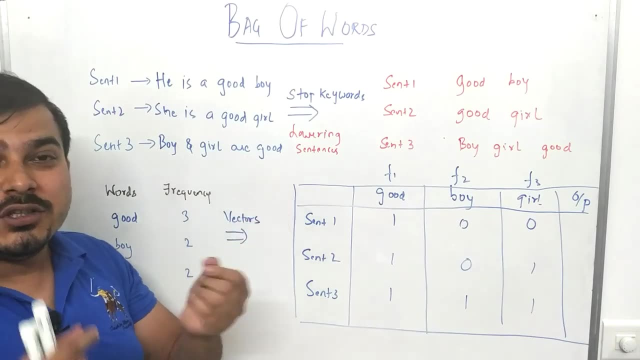 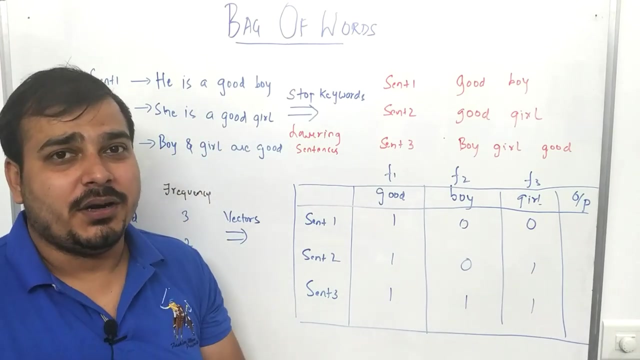 and this kind of data will be present a lot, but these are not the major data. the major data is basically this: good word, boy, you know a boy, girl, good. so these all kinds of data are pretty much important. remaining words like he, she is a right, it is not that particular important, okay, so after. 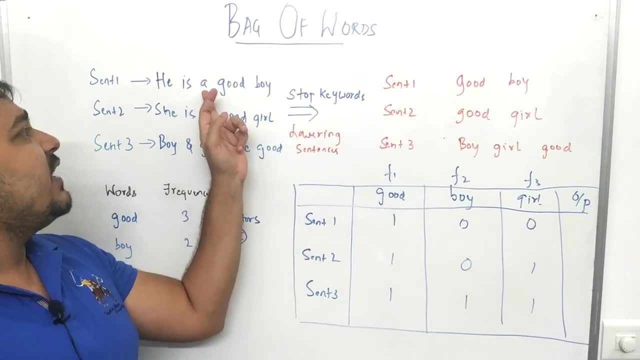 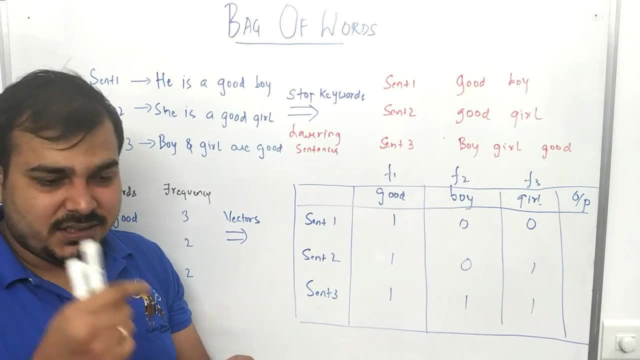 applying stop words. you know my sentence. you know all this particular words will get removed like is because: and again, if you, if you don't know how to do it, just see my next video in this specific playlist. the link will be given in the description. from there you'll be able to see how. 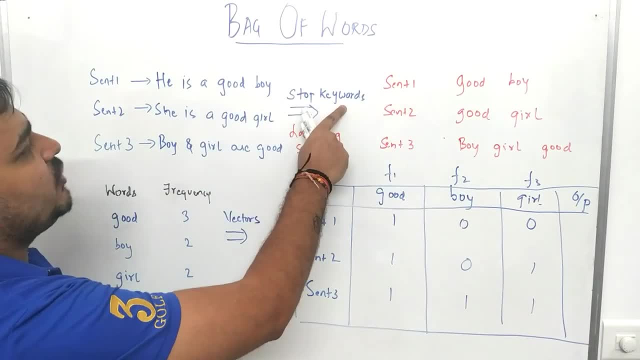 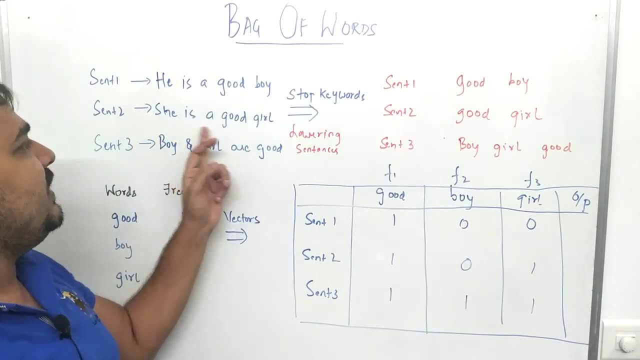 we can implement with the help of Python also. so after I apply stop words to this sentence in my sentence, one will become good boy. so here you see, he is, as gone. right sentence to: she is: there is gone. so we are having good girl. so over here in sentence three, boy and girl are good, oh yeah, and. 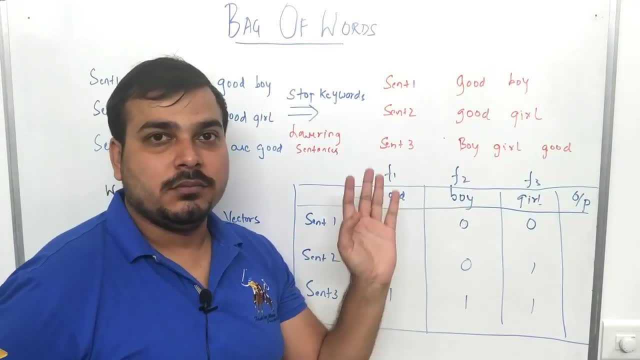 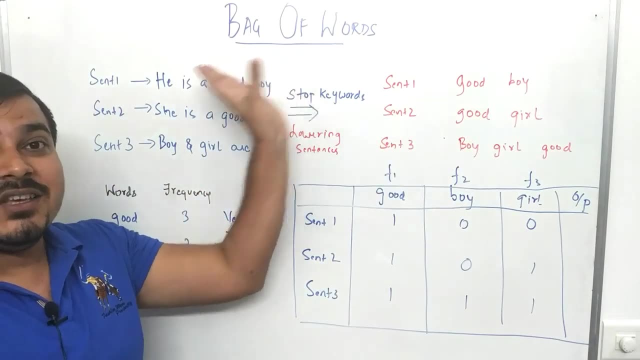 an hour will go, so I just have three words: boy, girl, good, okay. so after applying stop words, we will be having this kind now, but our main name is that: how do we derive vector by using bag of words right, and that we are going to show you now. now I have this three. 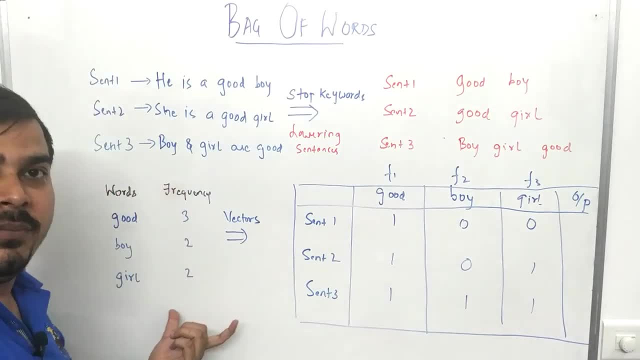 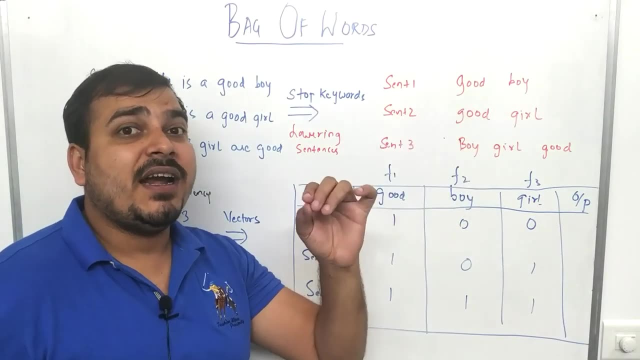 sentences. what I'm going to do is that I'm going to create a histogram- histogram from these three sentences. what does histogram basically mean? I will go and see for each and every word and I'll just try to find out. what is the frequency, what is the total count? 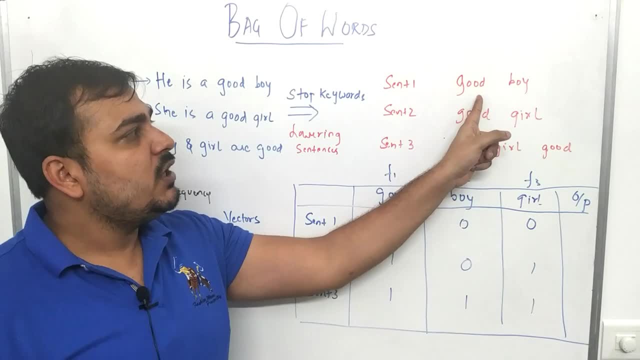 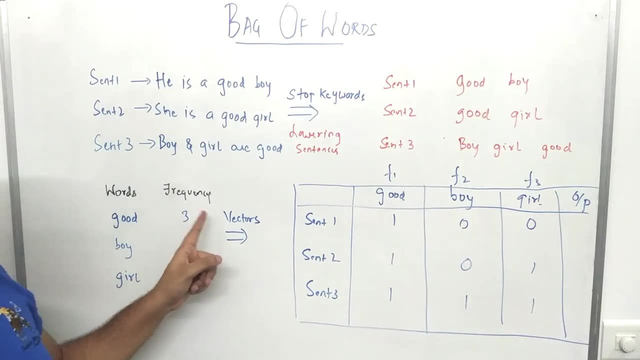 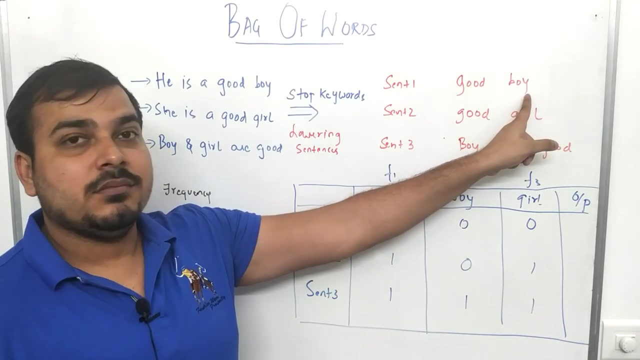 that it is present. suppose, if I take an example of good, good is present how many times? one, two, three, in all the sentences it is present. so I will increase that particular count to three. okay, so what I'm doing sentence is one, I'm taking good three. okay, boy, how many times it is present. see, I've just going sentence by. 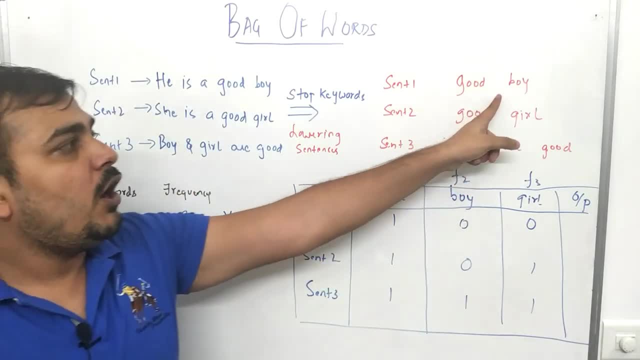 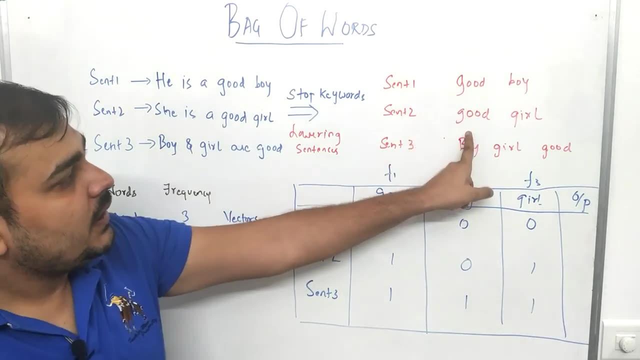 sentence. how many words are they? I'll just try to find out the frequency. so boy is basically present two times. you can see one and two in sentence. one and sentence. so I have incremented the count to two. then you can see again. good is there? girl is the new word. so I'll write girl. I'll try to. 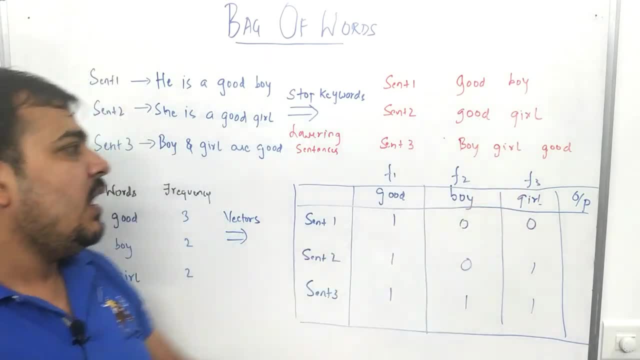 find out what is the count, how many times girl is present. one and two again, and the sentence three is basically having the same word. so I'll keep it like that, only so this three words have got derived from this and we have actually calculated the frequency. now remember when we are calculating. 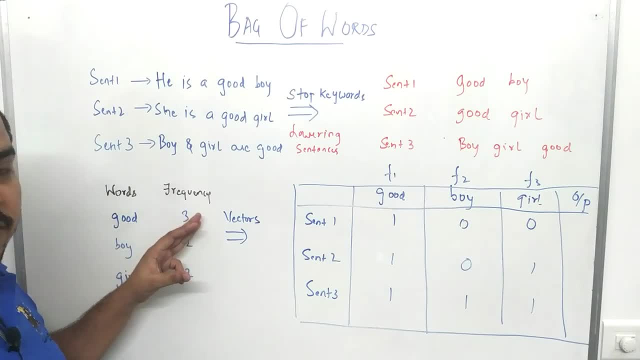 the frequency. they may be not in order, but we always have to sort from in the descending order. okay, so we need to sort this now. once we sort this, what we can do is that this all good boy and girl. now we are basically going to apply bag of words. so now this step is 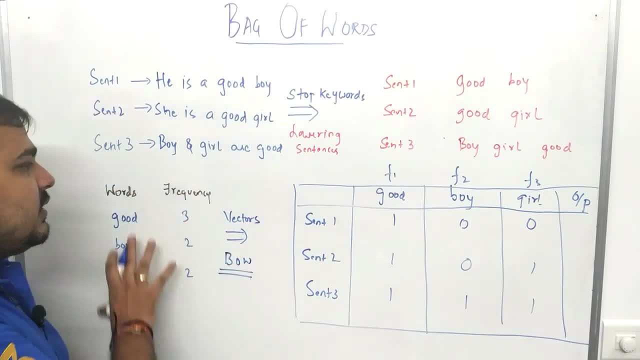 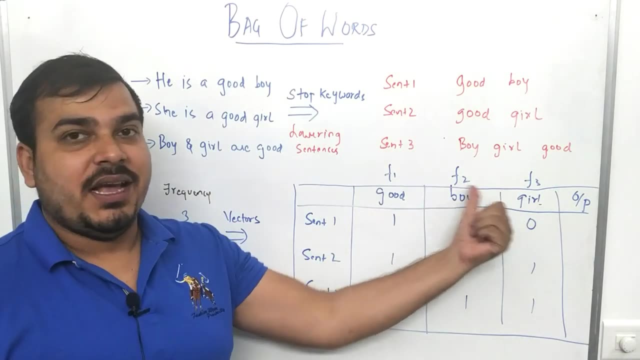 basically called as bag of words, where we are converting this representation into vectors. now this good boy and girl- I am going to write this as my feature- f1, f2 and f3. so here you have: good boy and girl. now I'll just consider my sentence one, my sentence: 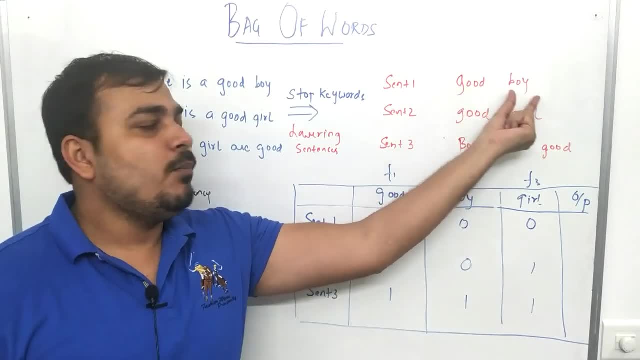 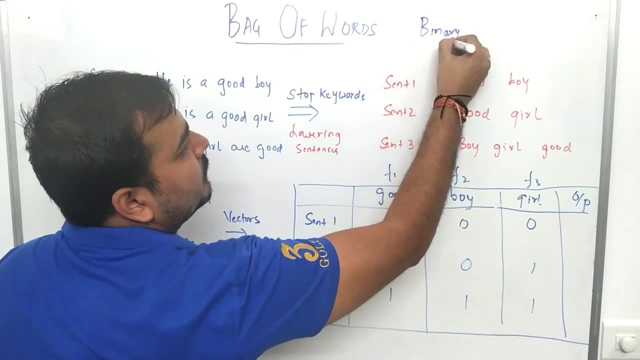 one is good boy right now. consider over here good, and boy is actually present. if I take an example and again remember, in bag of words there are something like binary bag of words and there is normal bag of word. these two example are there. first we'll discuss about binary bag of word. 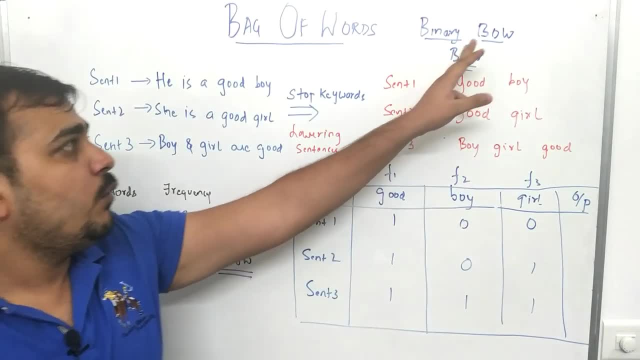 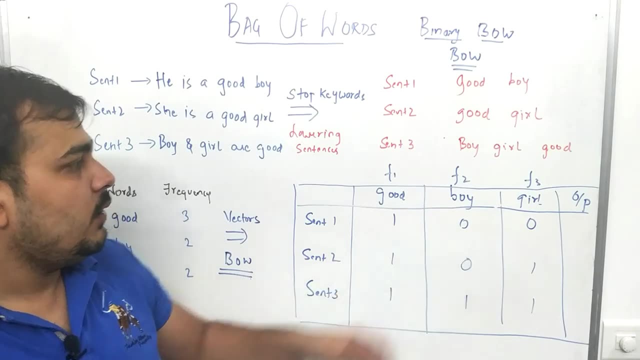 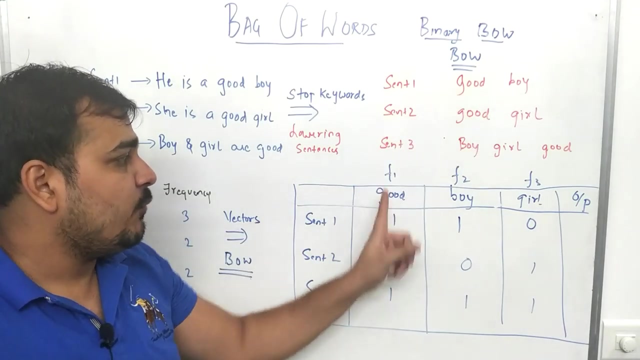 then we'll discuss about bag of word. now, in binary bag of word, what happens is that suppose in sentence one good is present, I'm just going to say it as one. if it is not present, then suppose over here, okay, over here, boy is also %, we will make it as one, okay, right. so if the word is present, I am. 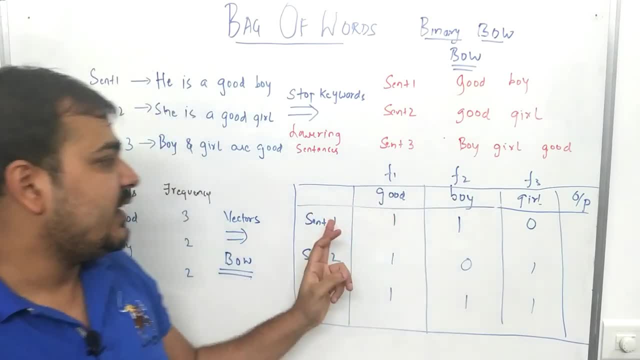 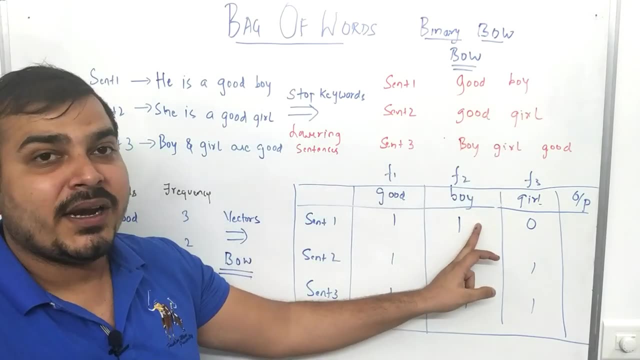 going to put it as one. if the word is not present, I am going to put it as zero. so in the sentence one you can see good is present. so I'll just go and look on the feature here. good is there, so I am going to make it as one. boy is there, I'm going to make: get a girl. 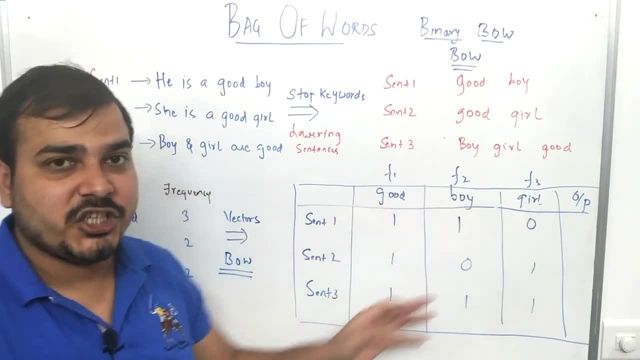 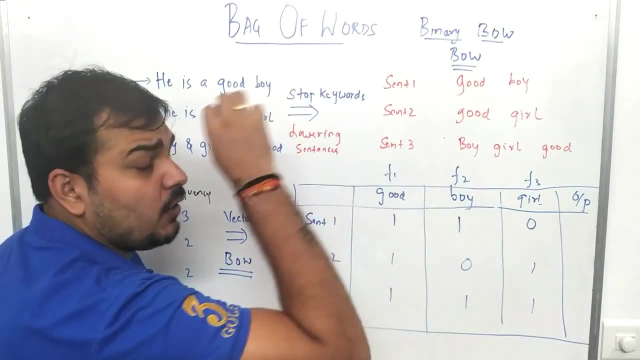 is not there, I'm going to make it as zero. so this is how my representation is there. now, understand this. this: this whole sentence is represented by 1 1, 0, and in binary bag of words we either have one or zero. okay, now in sentence two. in sentence two: 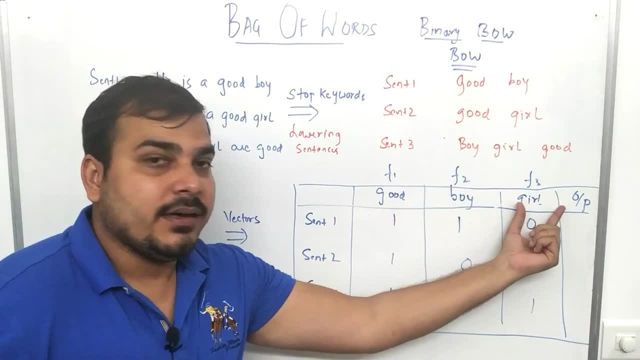 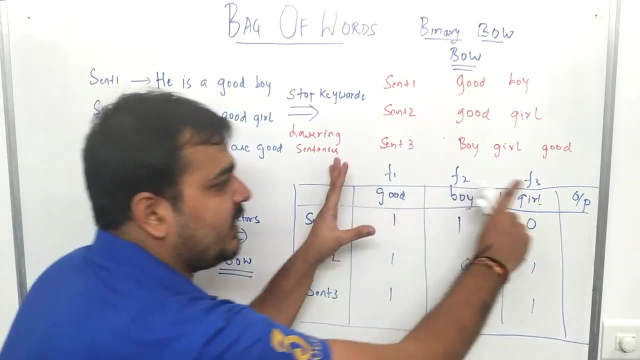 i have good and girl right. so good is over here, girl is over here. now i have one zero, one right, and similarly, for sentence three, i have one, one, one. now, understand that this is vectors, this is vectors. now, the most important thing is that. what is the second bag of words? now? suppose, imagine, 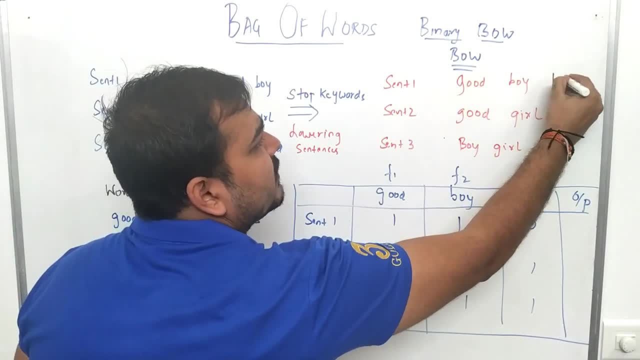 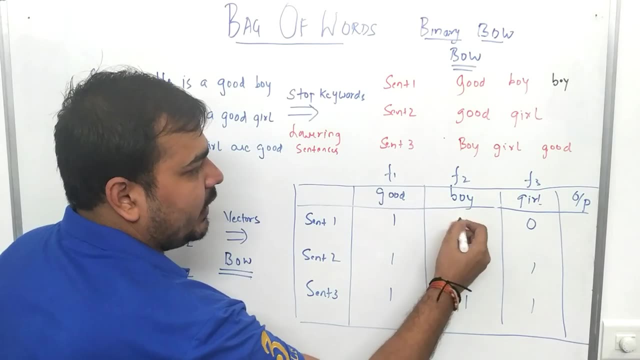 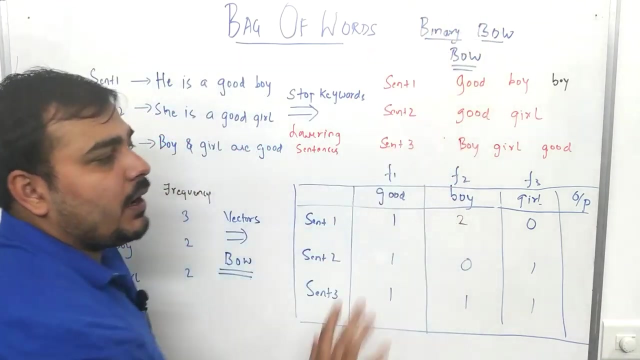 that i have good boy. one more word is there, suppose boy? okay, now you can see that boy is getting repeated two times. so when it is getting repeated two times, i can actually increment the count and make it to two. okay, so this is how you can actually use bag of words and binary bag of. 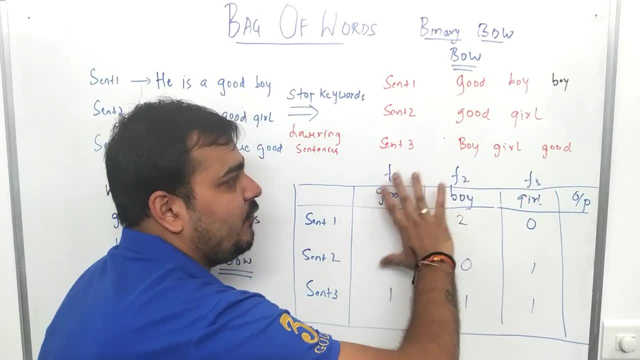 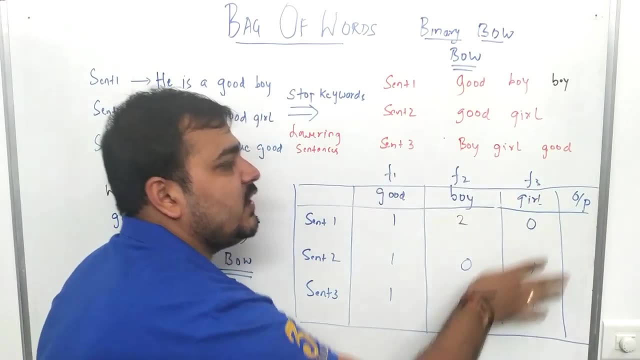 words, but remember, this is my features. this is my f1, f2, f3, right, how can i apply machine learning models? i'll also have an output column. so this f1, f2, f3 are my dependent feature. with this vectors, this will become my sorry. this is this: f1, f2, f3 is my independent features and this output feature. 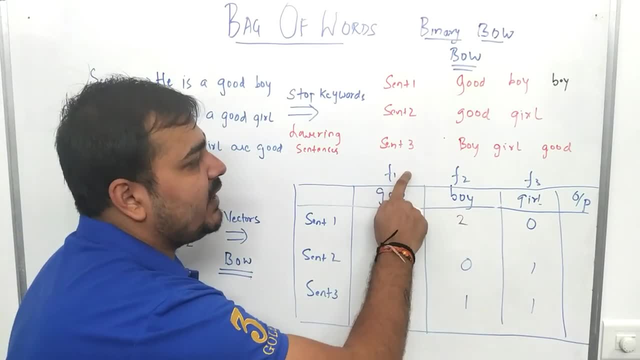 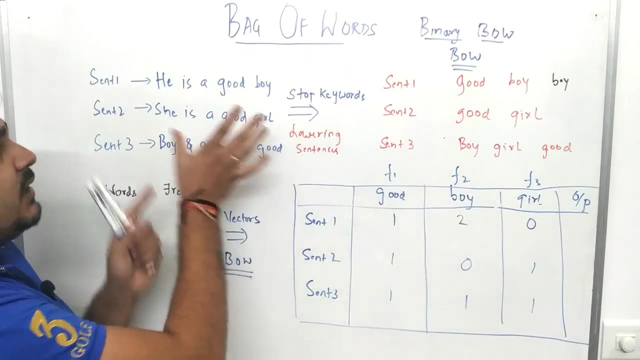 will become my dependent feature. so in my machine learning model i'll be training with f1, f2, f3 as my independent feature and my output feature, which will be there in this particular sentence. in my data set it will be there, right? this is just my input and i'll also be having an output column. so this is how my feature. 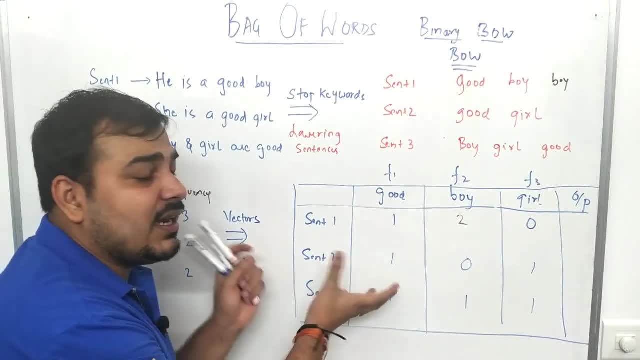 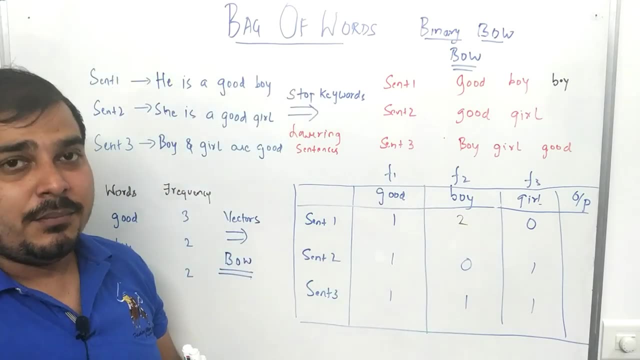 got converted into some numerical representation and now i can give this to my machine learning model and you know, and i can train my machine learning model and this is how bag of words actually work. but what is the disadvantage of bag of words? because we have better techniques. we have 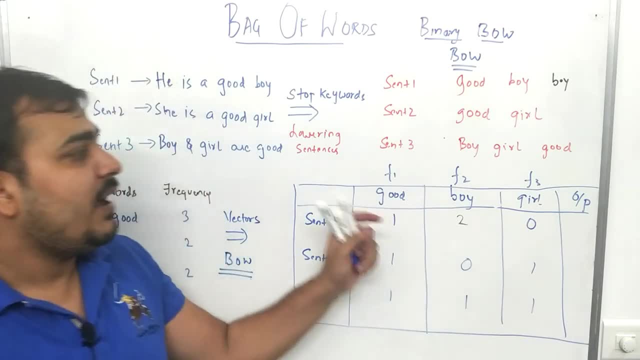 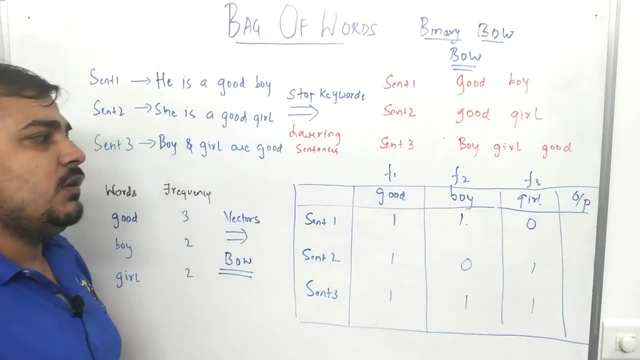 tf, idf. we have word to vec. what is the disadvantage of bag of words? because we have better techniques. what is the disadvantage of bag of words now, in this scenario? what you saw, guys, okay, i'm just going to convert that into the previous mechanism. now, here, what you have seen is that my values are: 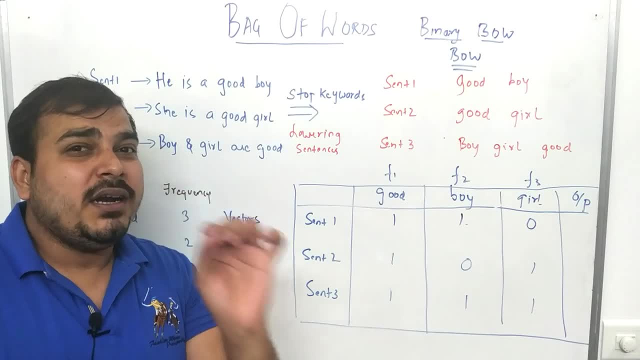 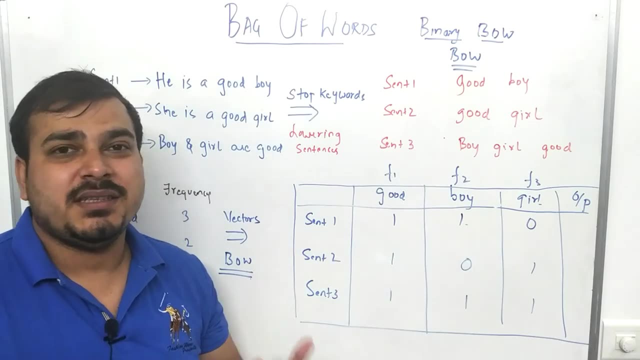 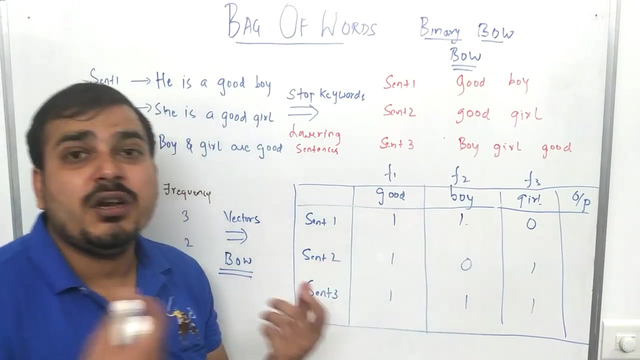 either one and zeros right. but one important thing to note over here i have this good: value as one boy, value as one right. both are having the equal representation right. the semantic of this particular words are almost same. we are not able to derive which word is much more important. 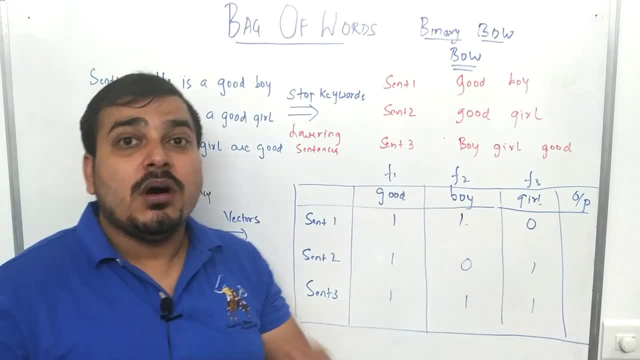 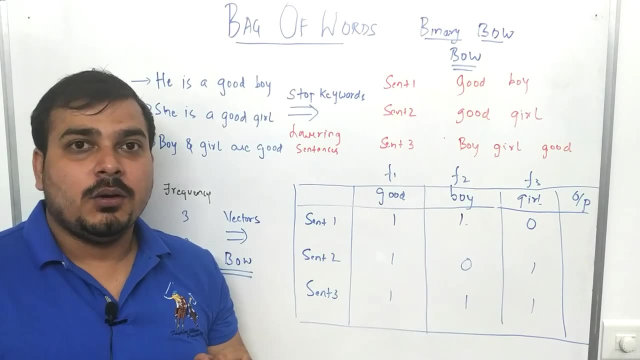 in sentiment analysis. the major thing is that we should know that which word is more important, like in this particular case, good should be important. suppose i take an example. uh, he is intelligent. okay, over here, intelligent is a major word. we need to try to give more value to that intelligent word. 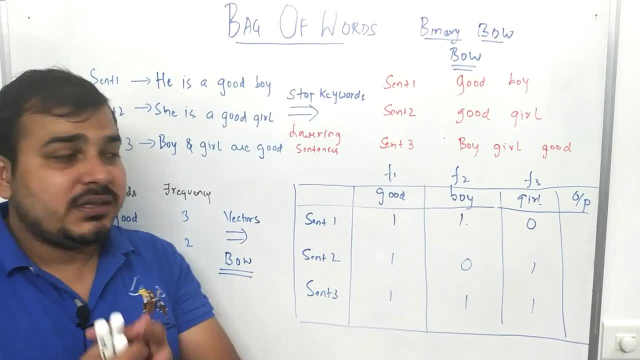 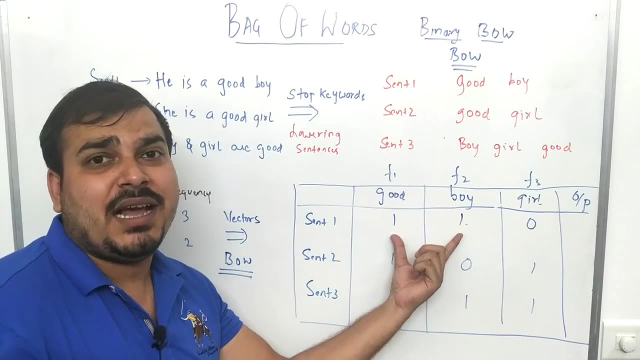 to actually derive a sentiment analysis. right, so that particular case. here you can say either we are getting ones and zeros. these two words has the same representation, right? one one, i'm just having this one one. there's no much more meaning to this one one. right so in this particular case, 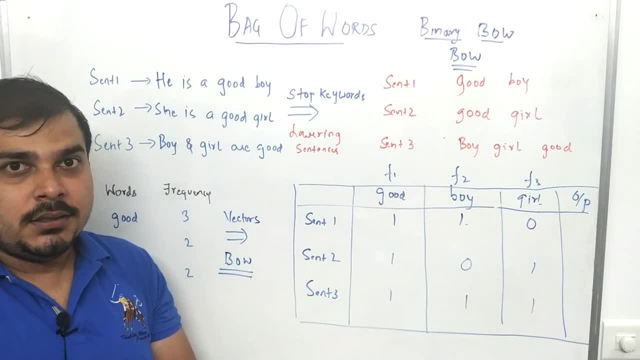 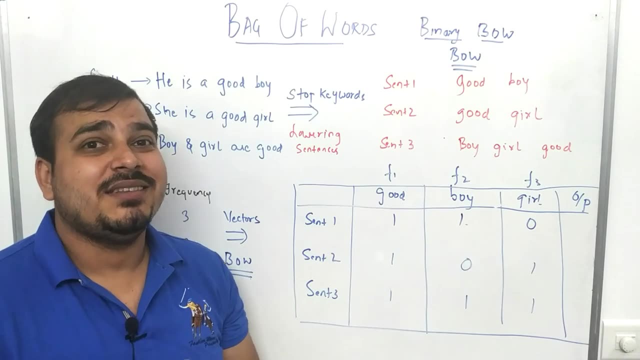 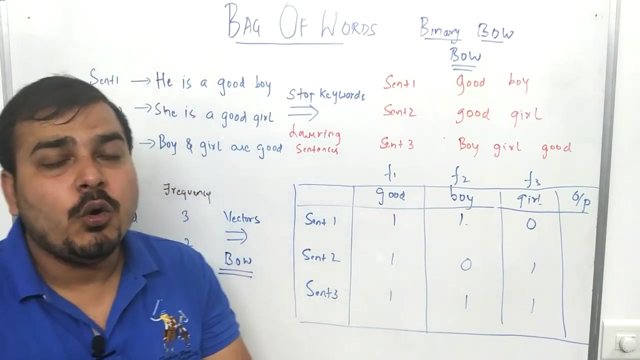 we have the same meaning out of it, right, they are given the equal weightage, right. so this is the major disadvantage of bag of words, and in order to solve this, you basically have something called as tf, idf, which is also called as term frequency and inverse document frequency. so we will try to